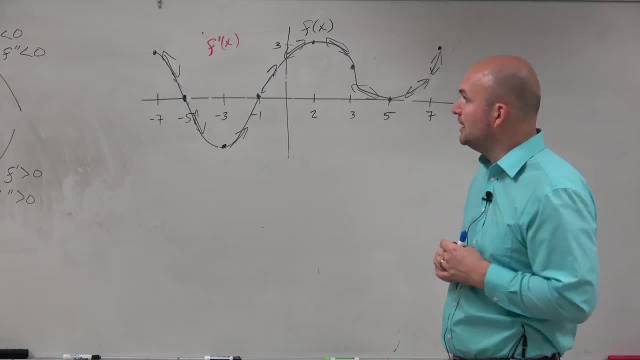 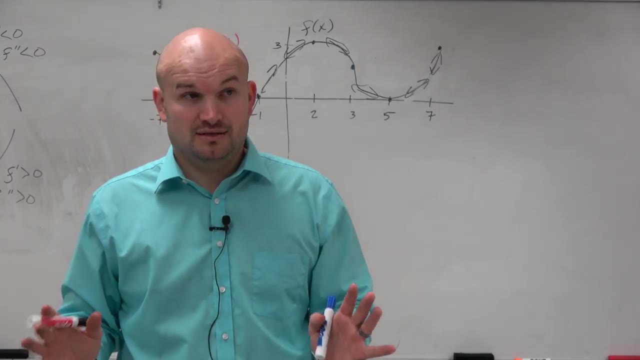 So let's pretend everything is. let's look at f prime of x Now. remember, f prime of x is talking about the slopes of f of x, correct? Yes? So if we're going to talk about f prime of x, 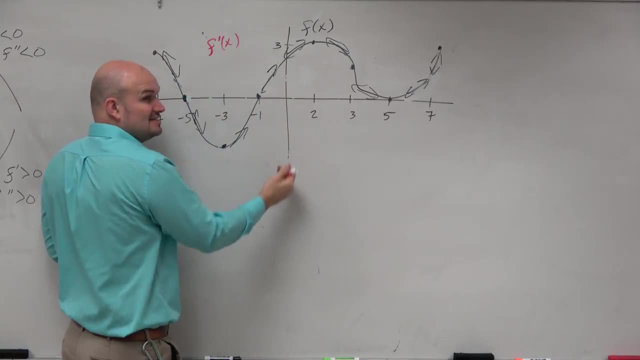 if we're talking about values of f, prime of x are less than 0, that means the slope of f of x is less than 0. So look at these slopes- Negative, negative, negative, right- And then it changes from negative to positive here. 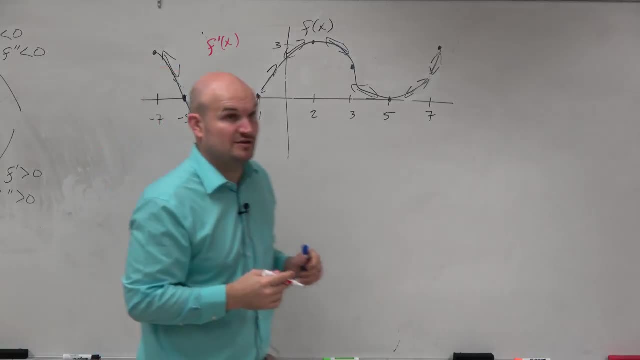 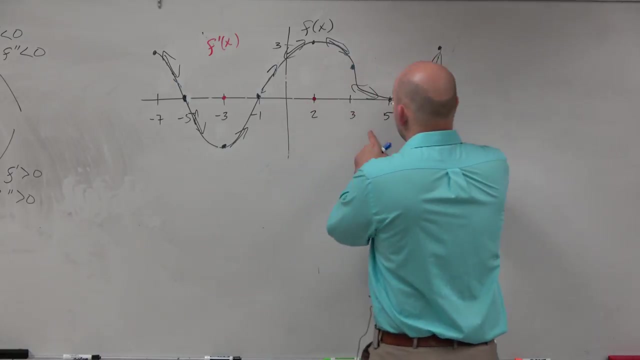 at 3.. So that means that's going to be a critical value. Where f of x is equal to 0, that's a critical value. That's a relative extrema. Then it also changes at 2, and also changes at 5.. 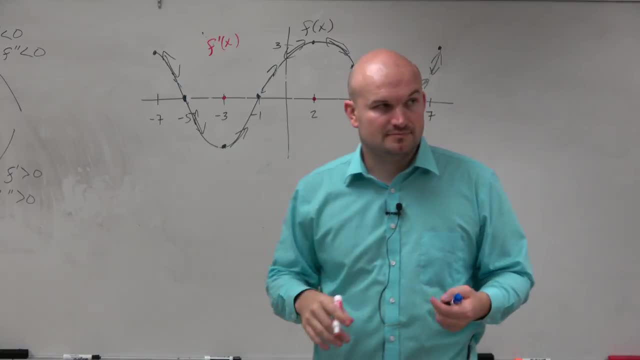 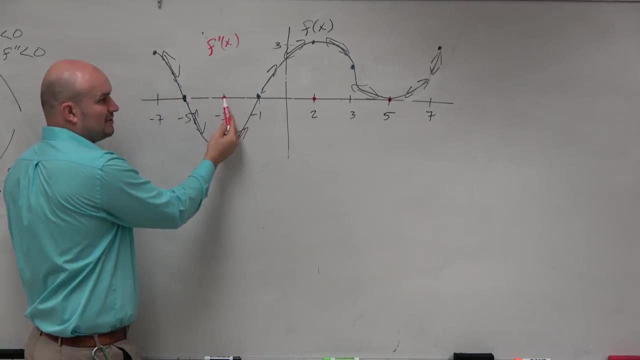 It changes from a negative to a positive. So again, we have no idea what the graph looks like. We're just estimating, We're just sketching. So from negative 7 to 3, we have a negative slope right. So that means my f prime of x needs to be negative. 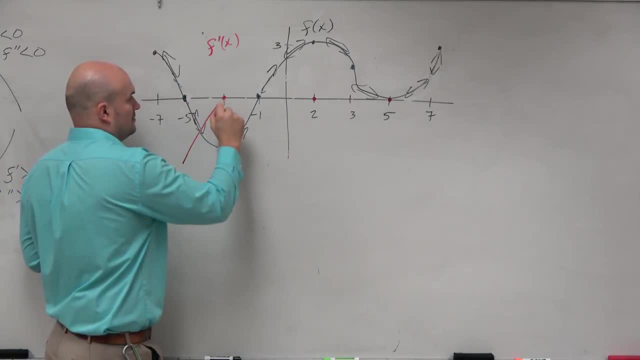 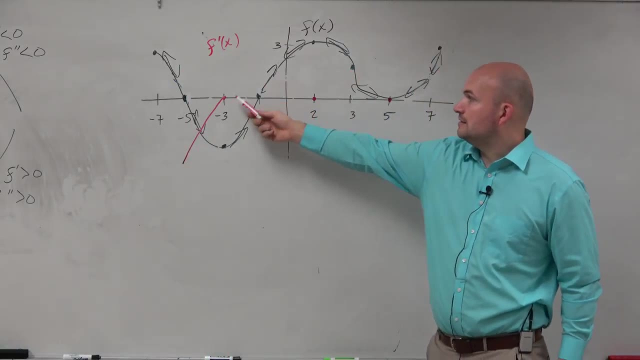 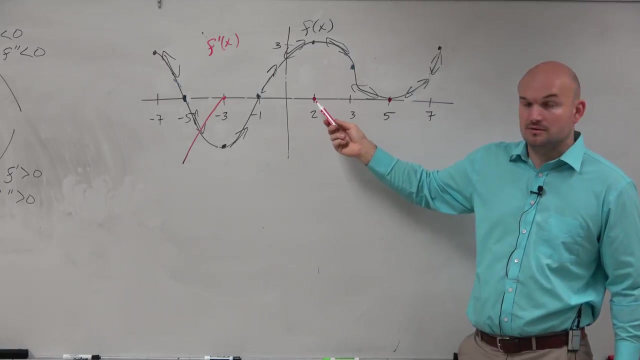 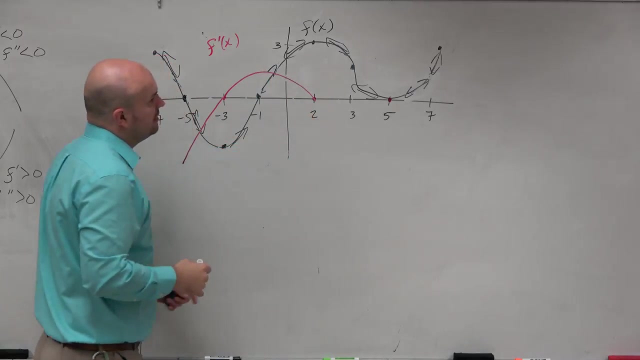 It needs to be negative. So we're changing from there. Then now it's positive from negative 3 to 2.. All right, All right, All right, Yes, Do you guys agree? No, Don't agree. So it's going to be positive from there. 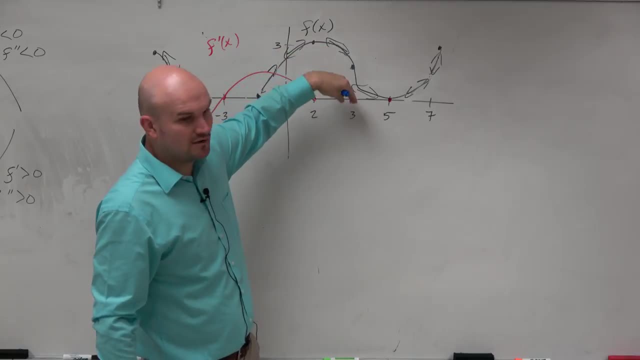 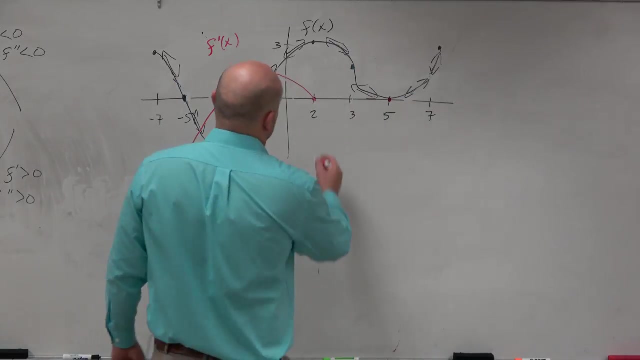 And then from 2 to 5, you can see the slopes are always negative, right? So from 2 to 5, we're going to be dealing with a negative, And then we can just draw something like that, OK, So the one thing I want you guys to notice: 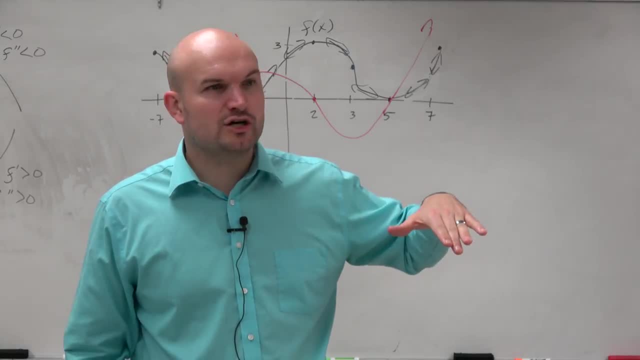 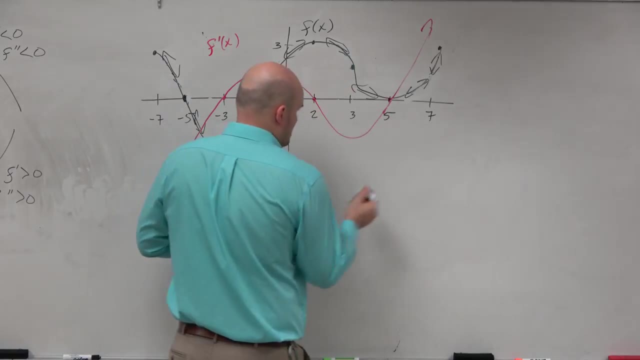 when you're going from f to f, prime notice how we kind of lost a turning point. right, We lost a turning point And again that kind of makes sense, Like if you had f of x equal to x. to the fourth: 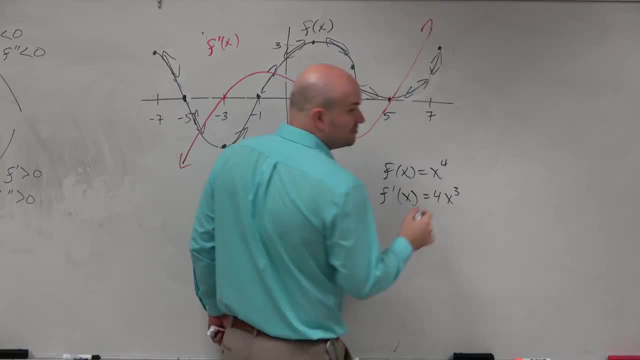 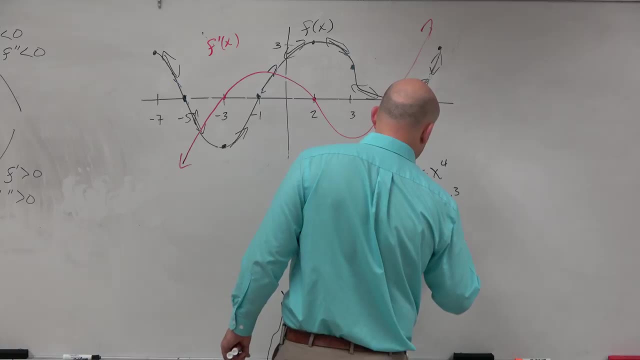 and then we do f prime of x. well, now we're leading at 4x cubed right, So we're losing a curve, We're losing a turning point And then, if we did f double prime, we're looking at 12x squared right. 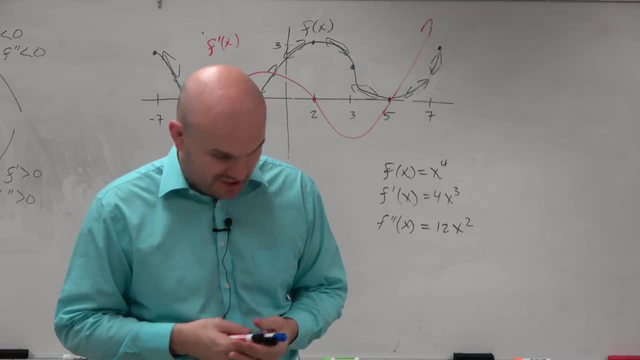 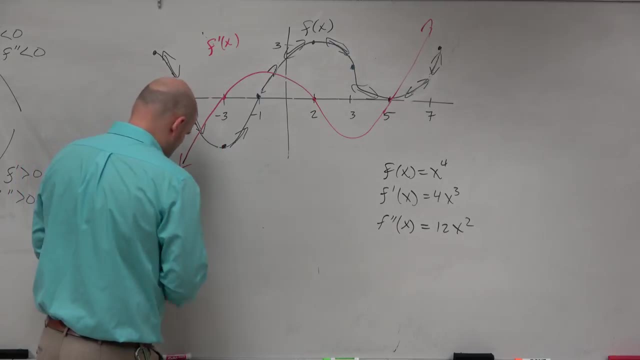 So now we're going to have a turning point. Now what we want to do is look at when are the slopes changing? So we look at the slopes changing, guys, And we see that the slopes of f double prime of x. 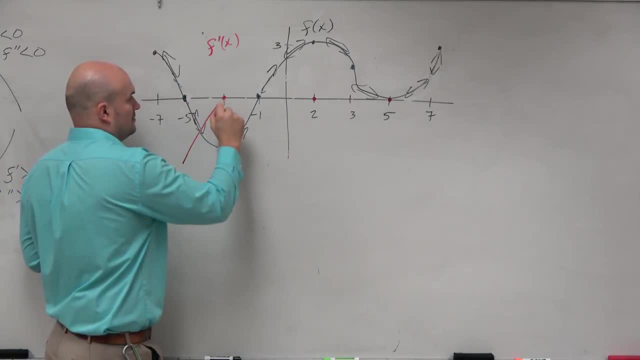 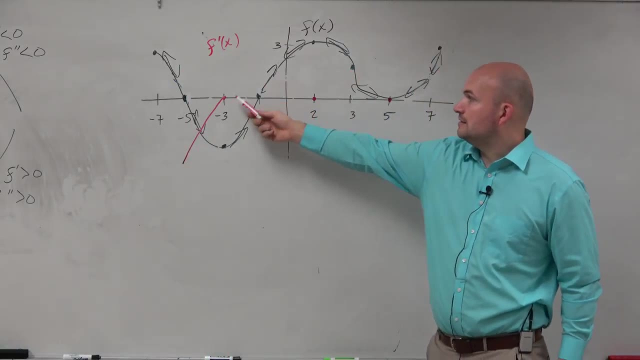 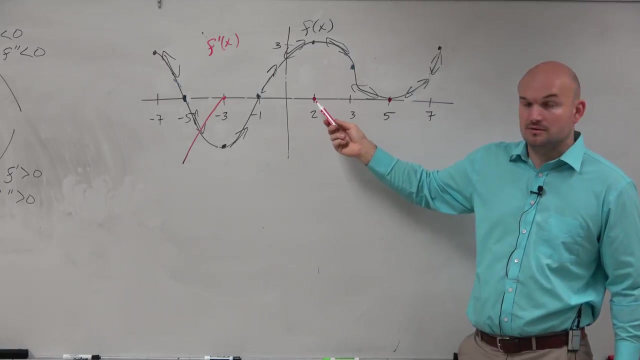 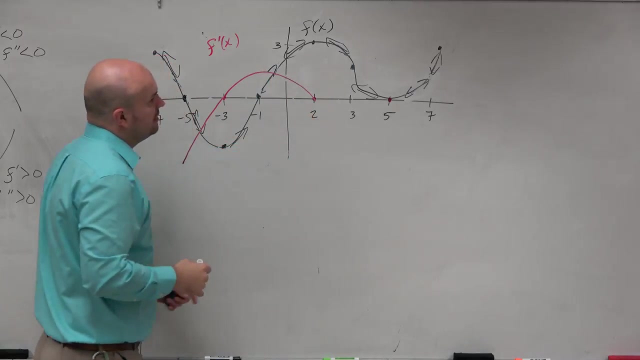 It needs to be negative. So we're changing from there. Then now it's positive from negative 3 to 2.. All right, All right, All right, Yes, Do you guys agree? No, Don't agree. So it's going to be positive from there. 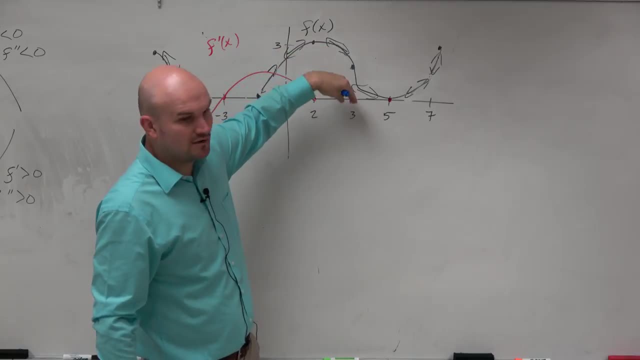 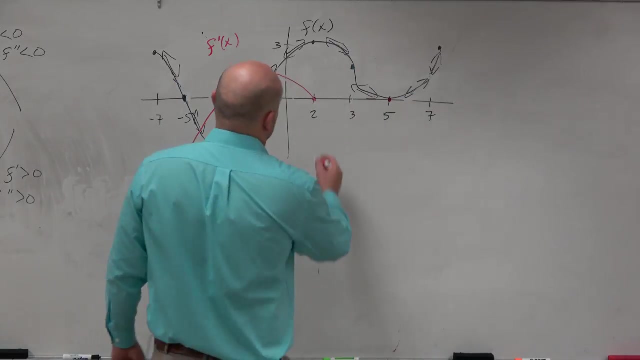 And then from 2 to 5, you can see the slopes are always negative, right? So from 2 to 5, we're going to be dealing with a negative, And then we can just draw something like that, OK, So the one thing I want you guys to notice: 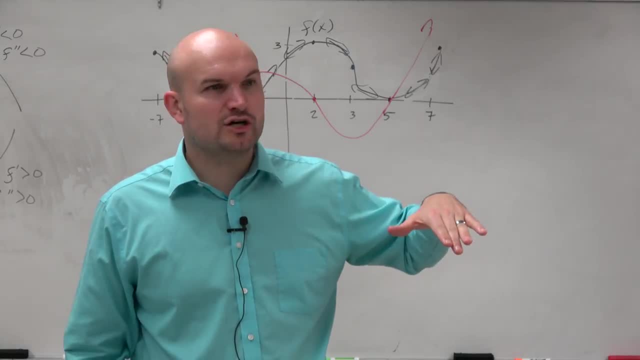 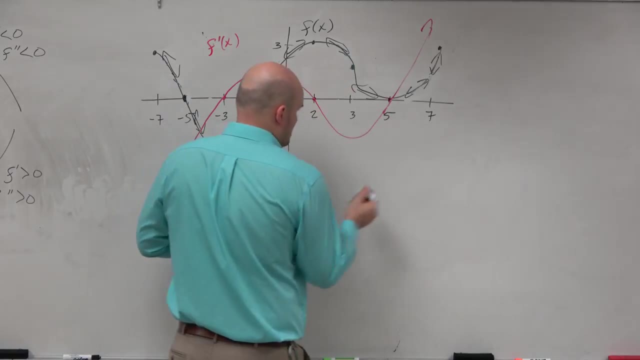 when you're going from f to f, prime notice how we kind of lost a turning point. right, We lost a turning point And again that kind of makes sense, Like if you had f of x equal to x. to the fourth: 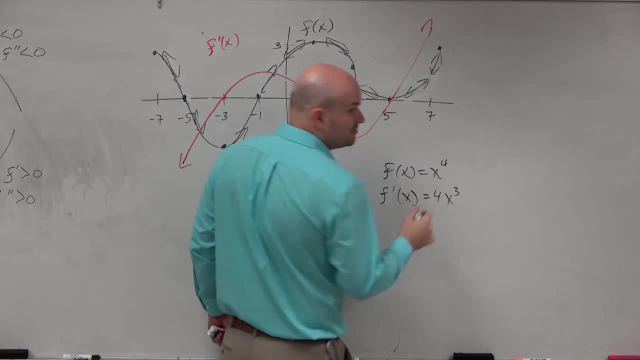 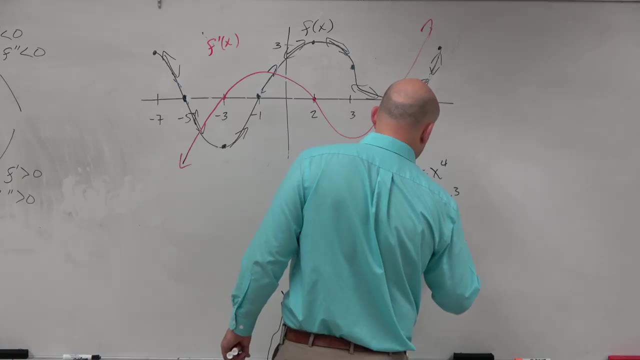 and then we do f prime of x. well, now we're leading at 4x cubed right, So we're losing a curve, We're losing a turning point And then, if we did f double prime, we're looking at 12x squared right. 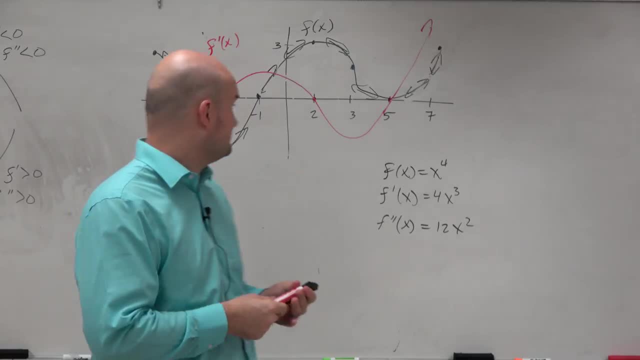 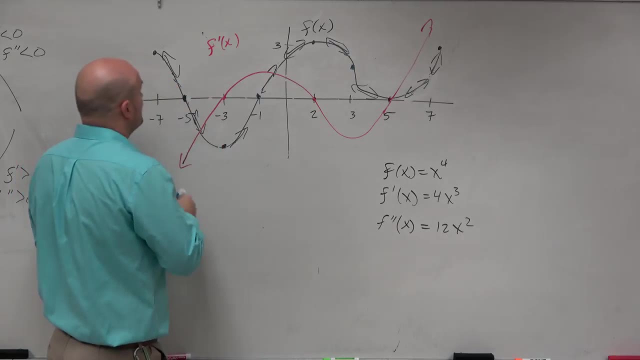 So now what we want to do is look at when are the slopes changing? So we look at the slopes changing, guys, And we see that the slopes of f double prime of x. so we'll do blue as f double prime of x. 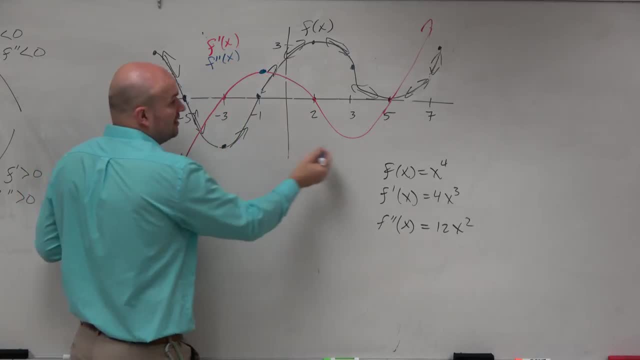 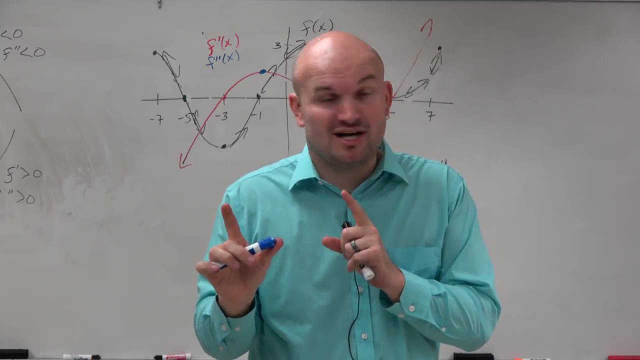 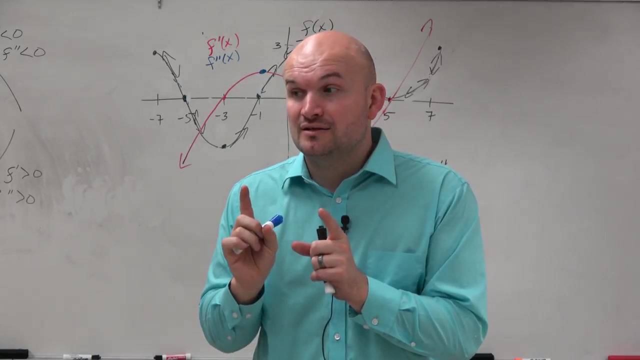 The slopes are changing right here and there. Yes, Also f, double prime of x. also tells us about concavity, And concavity tells us about what: Concavity, Concavity, Concavity, Concavity, Concavity occurs at the points of inflection. 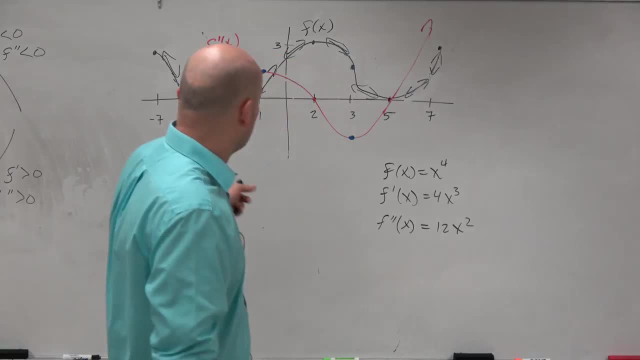 where the second derivative would be equal to 0.. So therefore, since it's changing here, these are going to be my new x-intercepts for my second derivative. Now look at these points on the f of x graph. Is that where the graph changes, concavity? 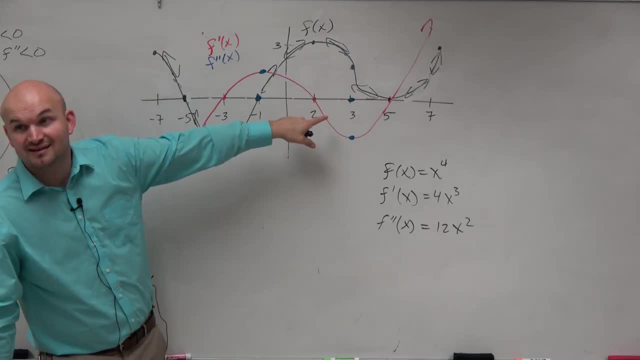 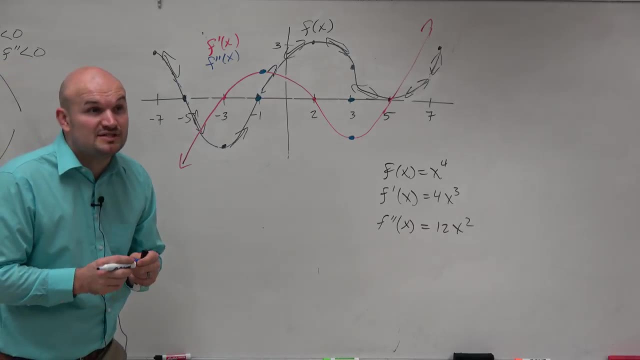 Does the black graph change concavity at these blue dots? It does. It does Right. So when the second derivative is equal to 0, that's the points of inflection. That's also where the concavity changes of f, of x.